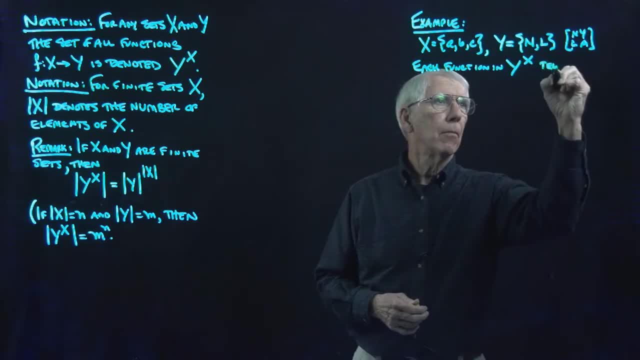 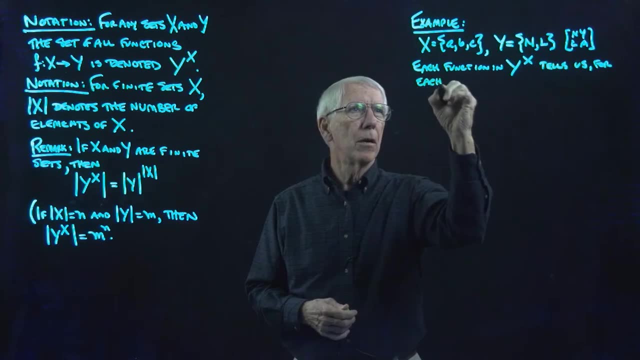 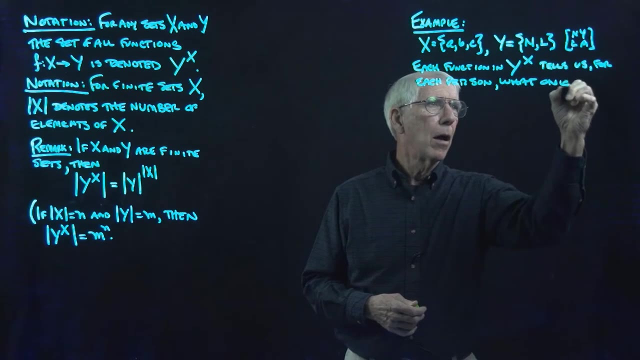 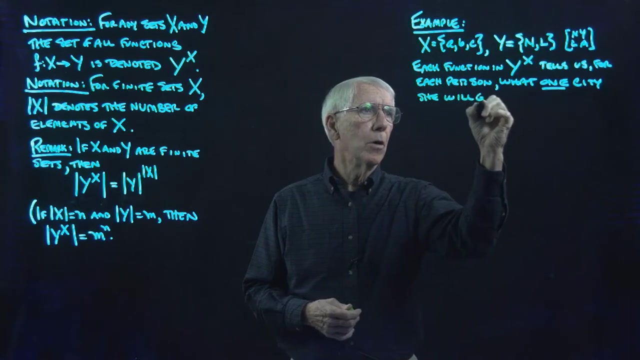 Each function in this set tells us, for each person, what one city she, let's say, will go to or was in or wants to go to. Doesn't matter, we'll say where she will go. So each of the elements of this is a function. 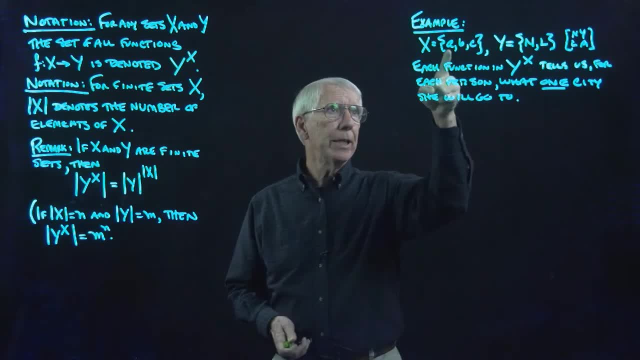 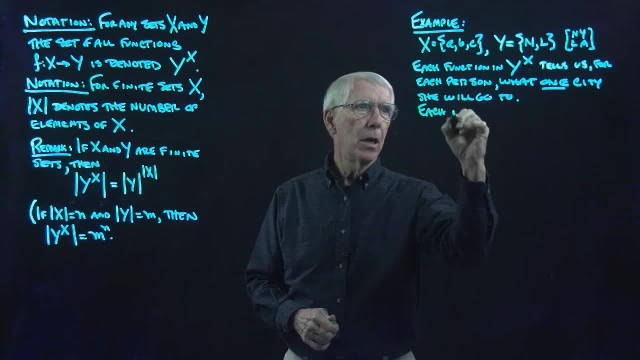 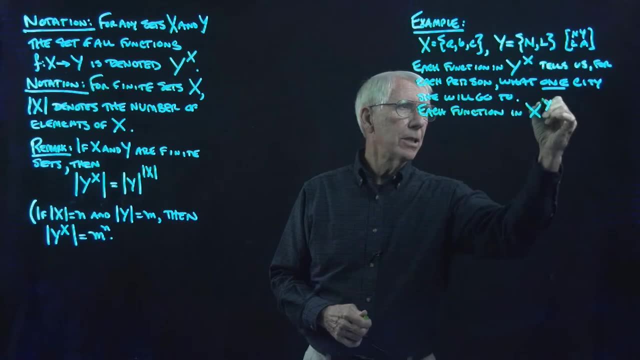 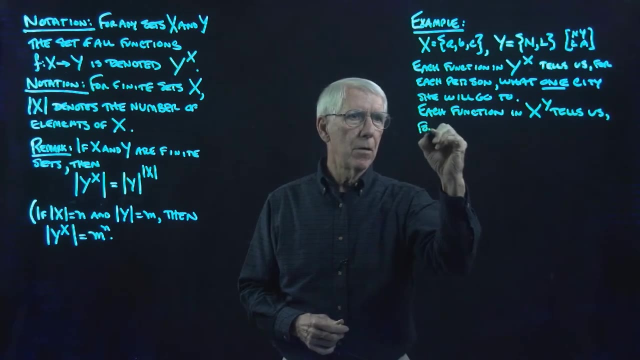 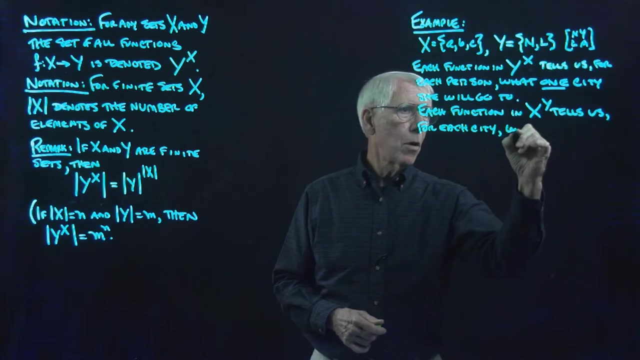 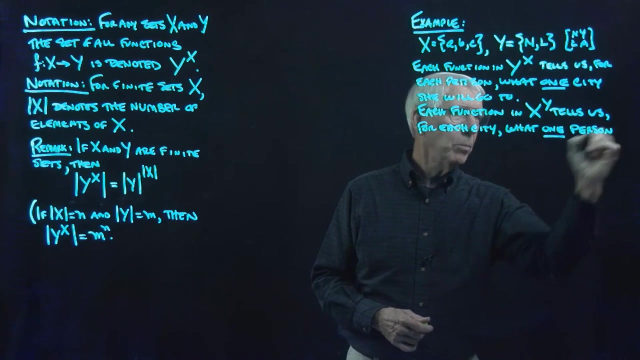 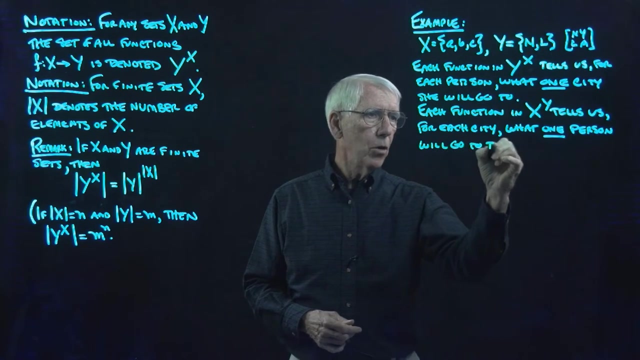 It'll go to And, of course, each function in X to the Y tells us, for each city, what it will go to And, of course, each function in X to the Y tells us what one person, which single person, will go to that city. 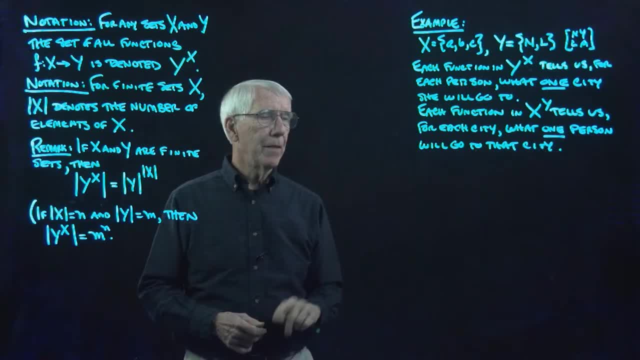 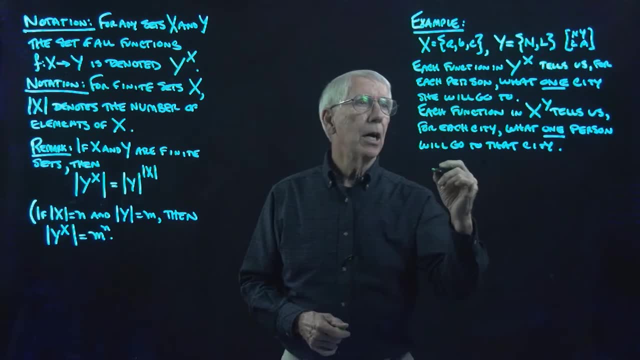 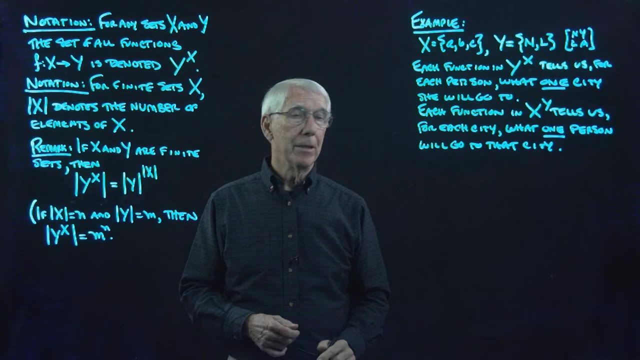 So in both cases here, emphasizing that a function has to assign only one thing, of course, to each element of the domain, And so in this case, of course, in fact, the fact that I'm interpreting this as people and cities isn't really the important point for what I'm going to say. 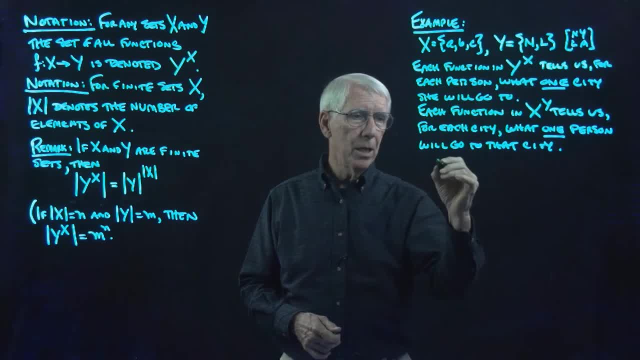 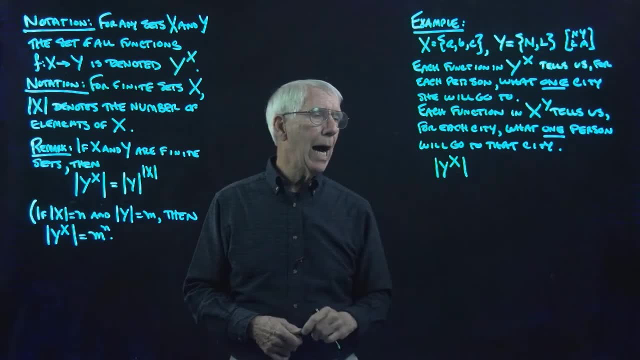 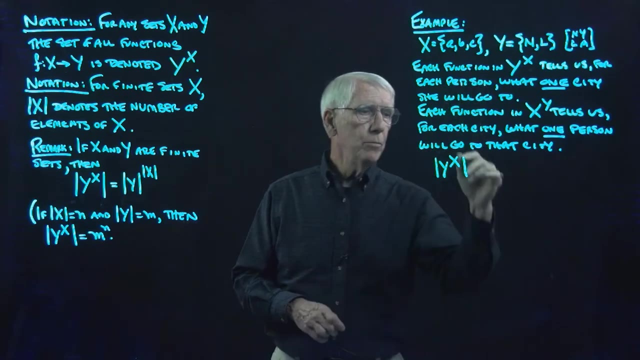 here. It's simply that there are three elements here and two elements here. So we know that the set of all functions going from x to y, that is, according to this, that is going to be 2 cubed 2 to the third, which is 8.. 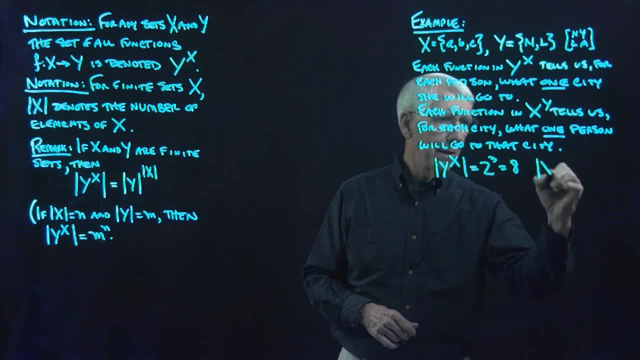 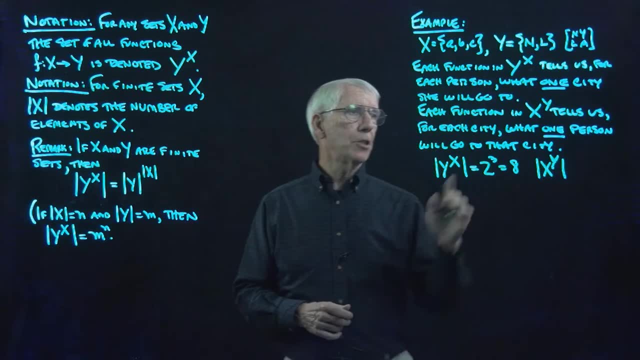 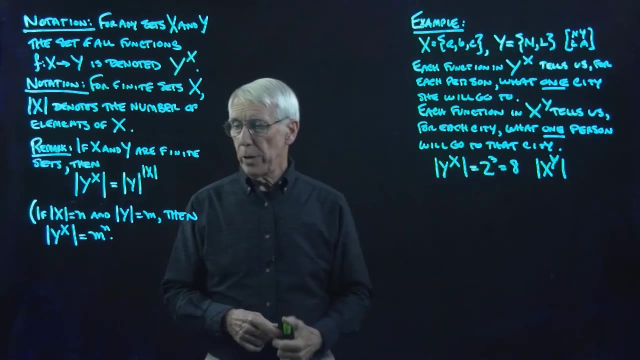 And we know that. I emphasize, these are sets, these are capital letters, the set of all functions from y to x. here that is going to be the reverse 3 squared. Again, we can just refer to what we did over here. 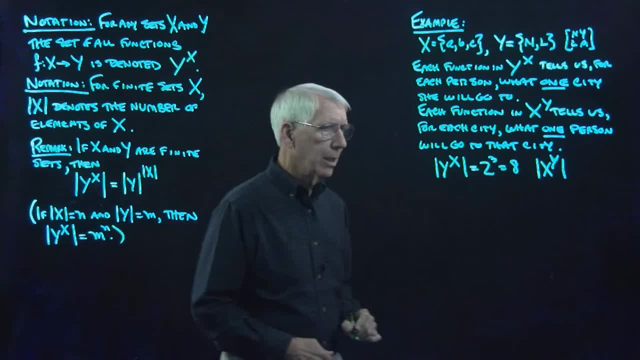 In fact I guess I should have put another parenthesis here, And so this is 3 squared, which is 9.. So there's nothing important about this example and it's not deep and it's not making any big point. 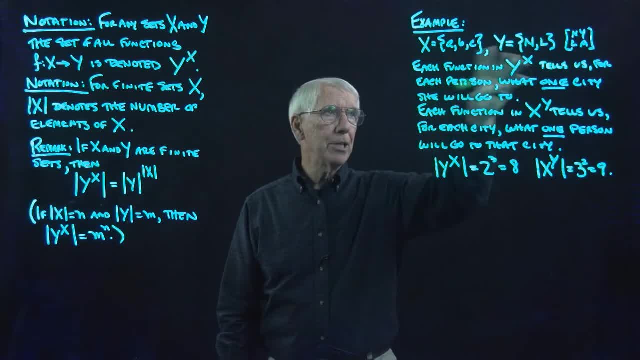 I just want to give a simple example with a finite, small, finite number of elements in each set and get an idea of what these sets might do and the number of elements in these sets of functions. Okay, so now let's look at another example. 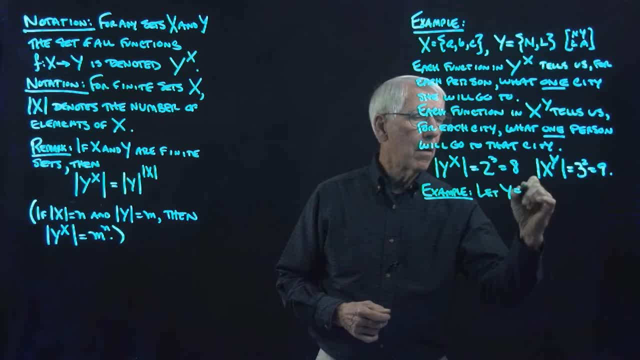 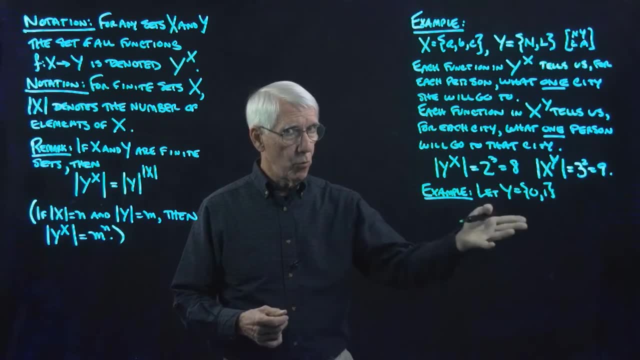 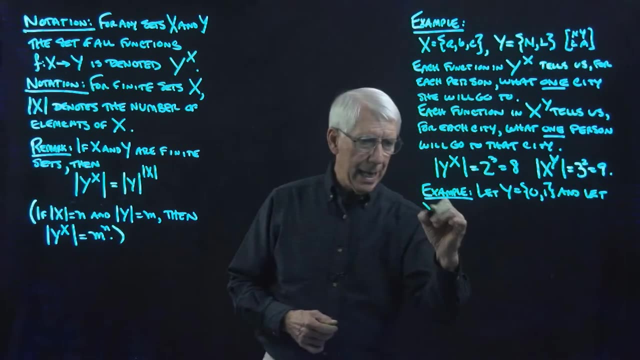 Let y be this 2-element set 0 and 1, and let x be the set 1 up to n, or in fact any n-element set would do. but this is a nice, convenient one. We can identify their n-elements. 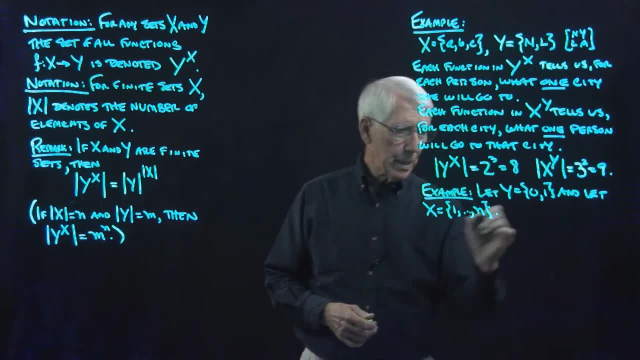 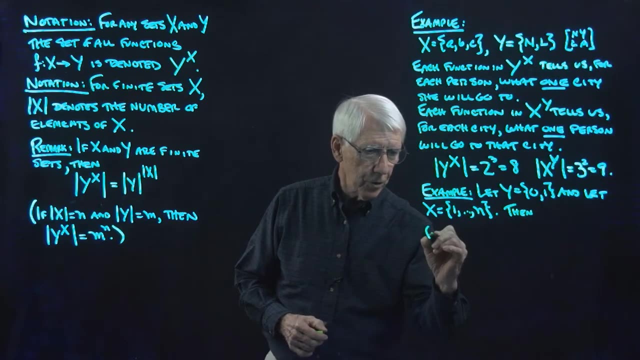 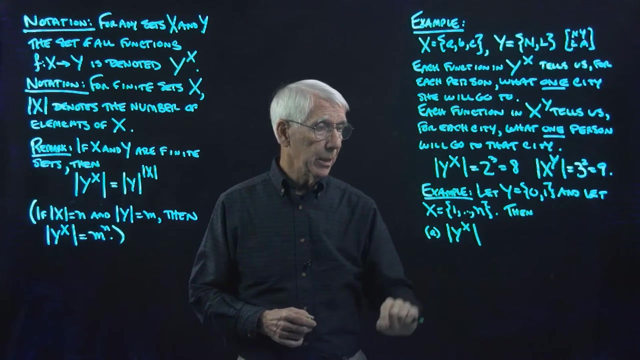 And they're the numbers from 1 to n, And then the. we have the following We have: first, let's note that the, the number of elements of y to the x similar to up here, is going to be 2 to the n. 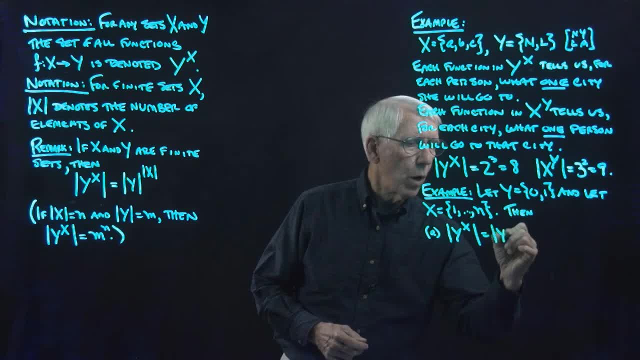 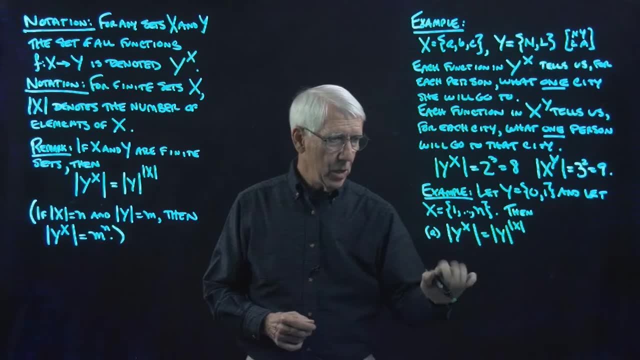 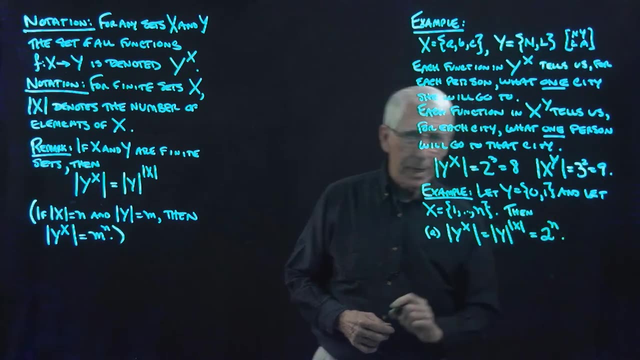 In fact, let's write that that is going to be number of elements in y: 2, the number of elements in x. so here these are actually numbers now, and that is going to be 2 to the n power. The other way round. 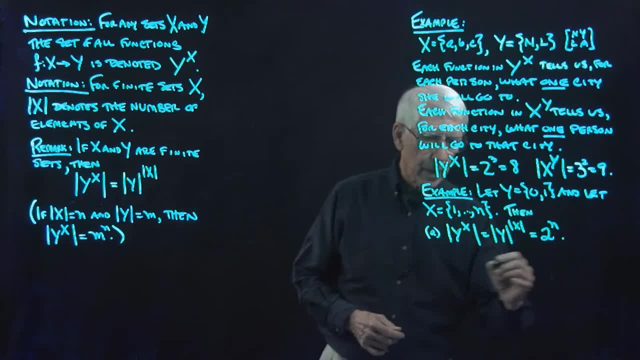 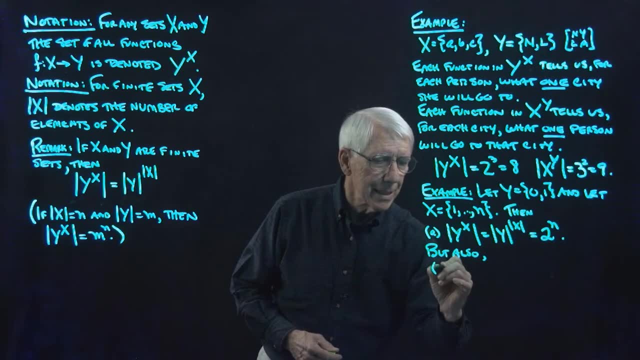 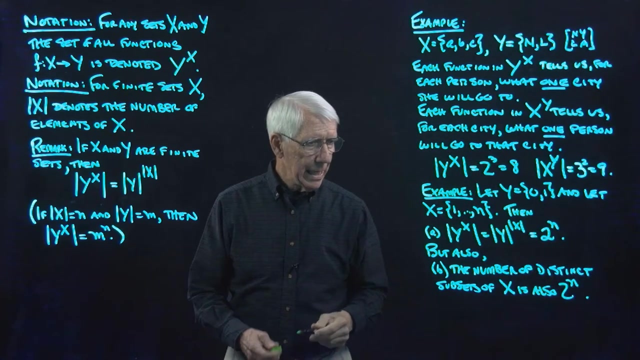 We're going to do 2 to the n. Okay, Okay, Okay. But also it's the case that the number of distinct subsets of the set x, as you can verify, is also 2 to the n. Maybe I'll make that 2 look a little more like that 2.. 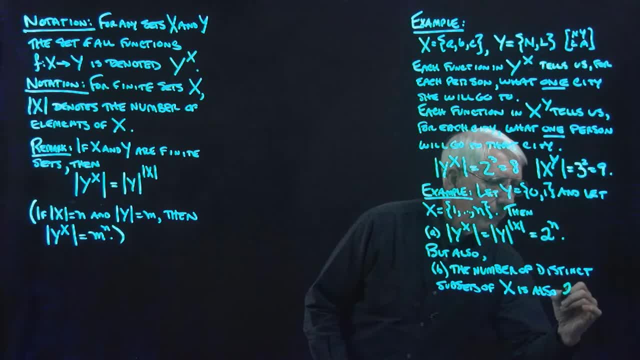 It doesn't look like z to the n, So I did that, and then I messed up the n, So let's fix this. Okay, 2. 2 to the n. All right, So you can say: well, okay, big deal coincidence. 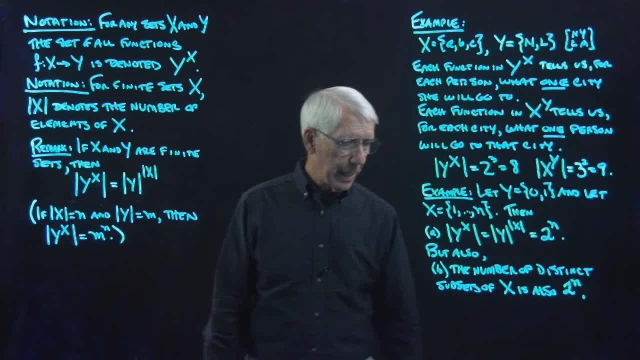 The number of things in here is 2 to the n. The number of things in here is 2 to the n. This turns out to be a kind of an important relationship between the two, and that comes from the idea of something called an indicator function. 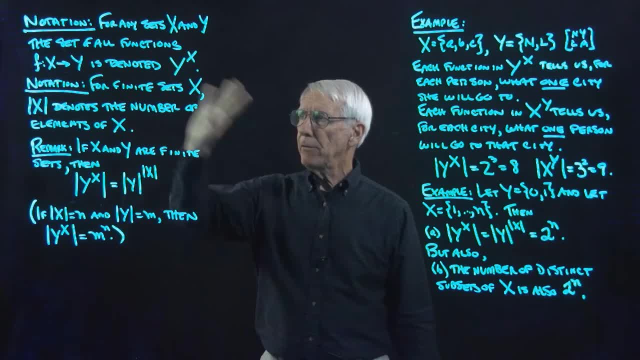 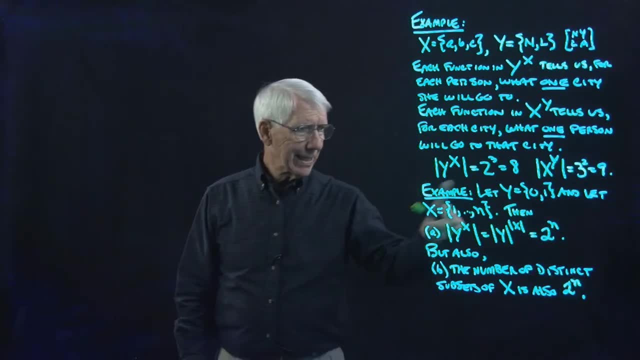 And we're going to put that Over here after we take off all the stuff over here so we can get some space. So this example down here: that the number of functions from this set x into the set consisting of just 0,, 1,. 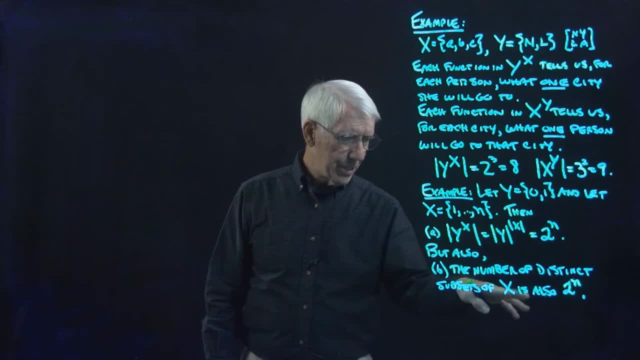 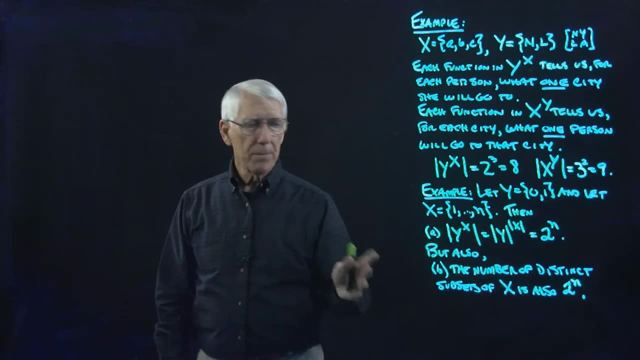 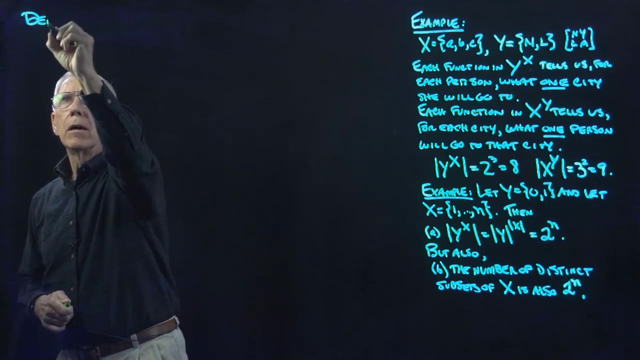 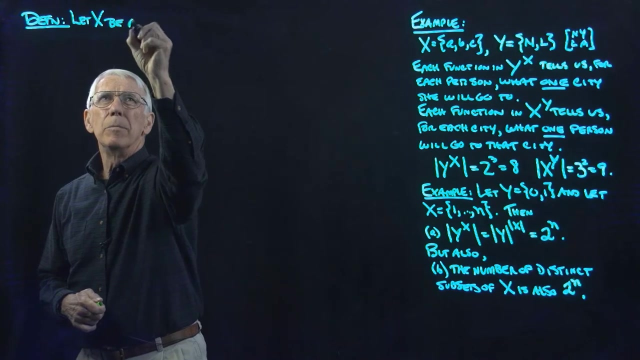 that the number of those functions coincides with the number of distinct subsets of the set x. that motivates a definition of something called an indicator function on the set x. So let's write that over here. Let's say: let x be any set. 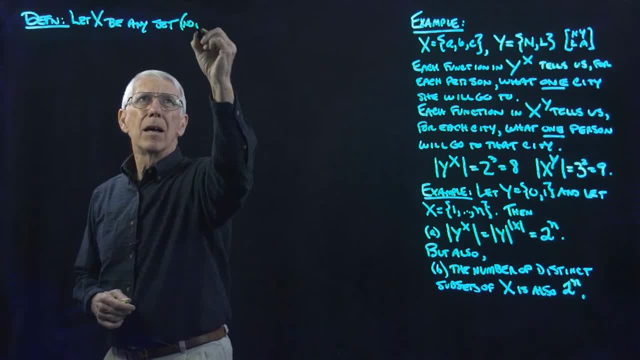 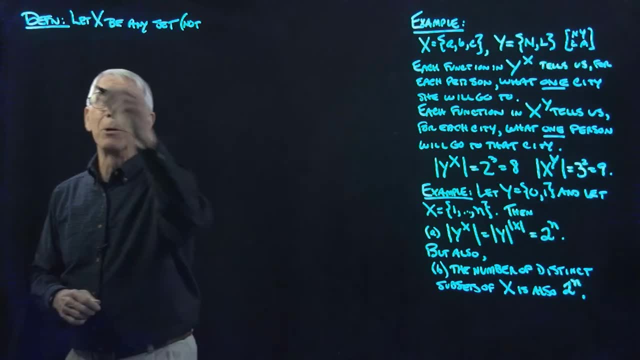 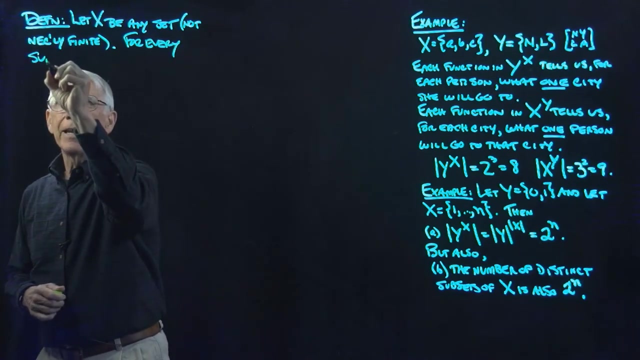 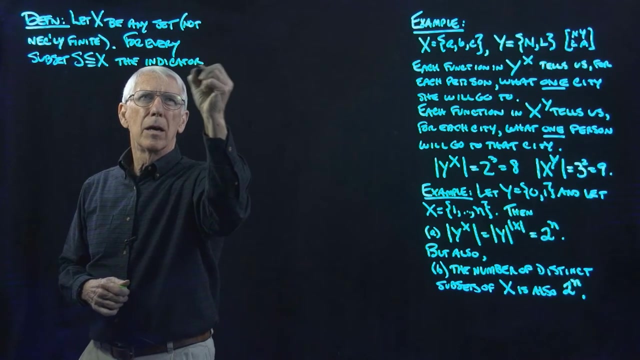 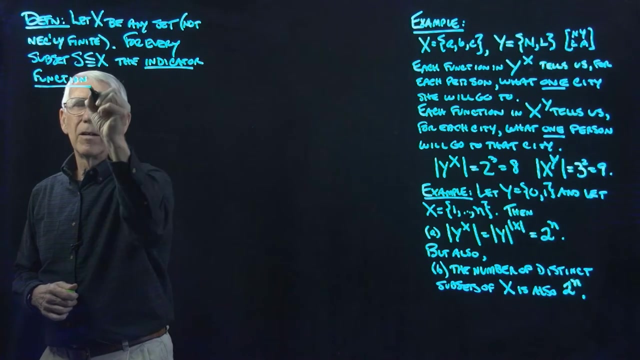 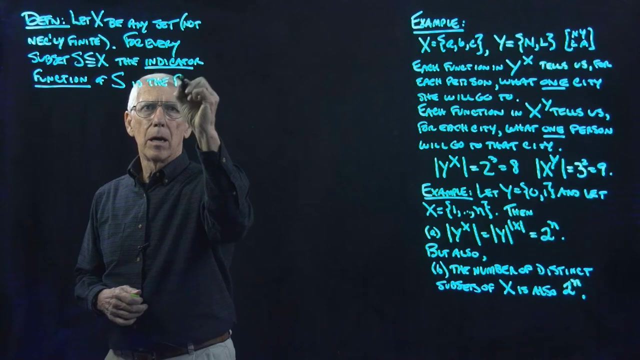 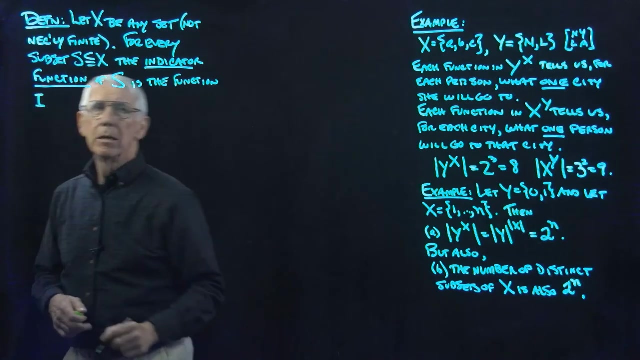 And now let me point out that it doesn't have to be a finite set like in the example. That's just a motivating example, Not necessarily finite For every subset s subset of x, the indicator function of that subset is the function that we denote. i for indicator. 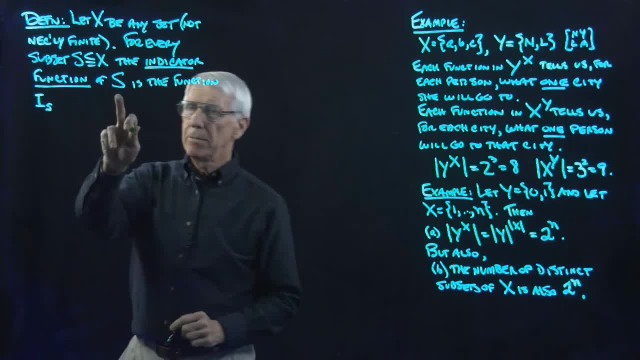 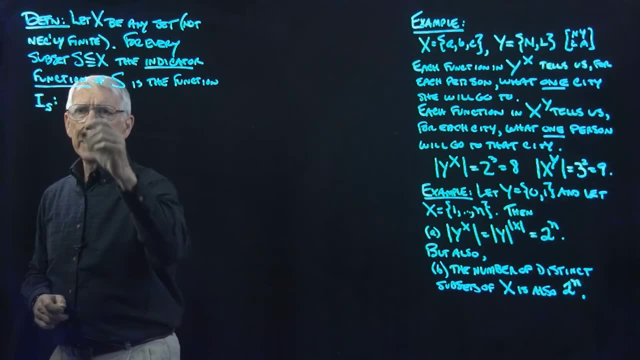 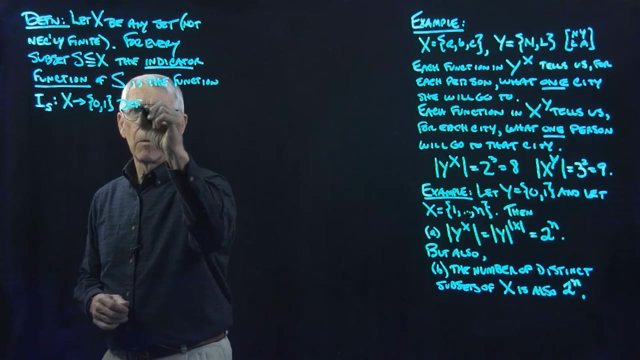 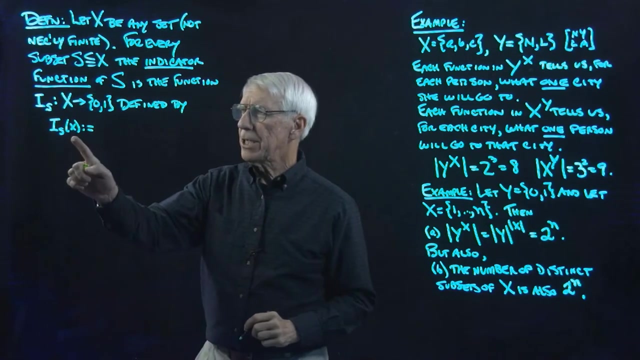 sub s, because it's the indicator function for the set x s from the set capital X, not the subset, the whole set into the set consisting of just 0, 1, defined as follows For each x in x, and I perhaps should have written that over here: 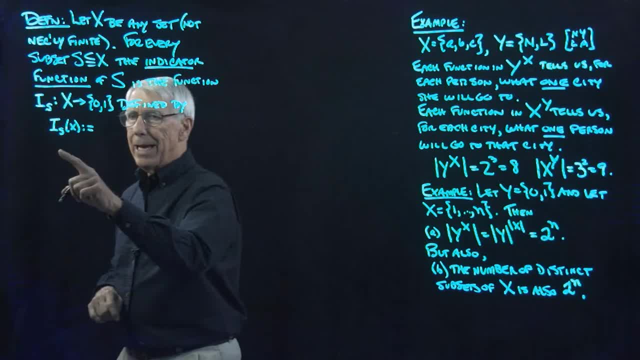 for every x in the domain i sub s something: x is 1 if x is in the subset s and 0 if x is not in the subset is. so you can see why we would parlicate an indicator extension, because the function of the sub set s is also different. 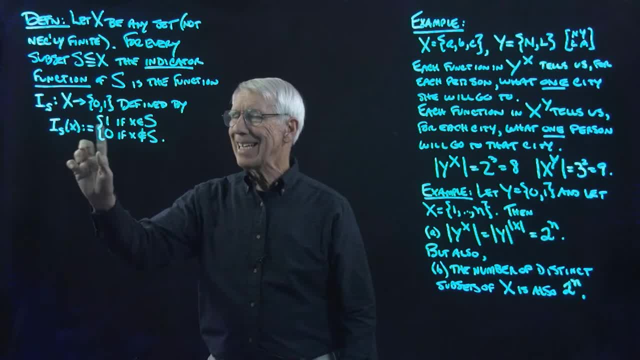 function. its value at every x indicates whether x is in the subset or it's not in the subset. So if x was the set of real numbers and s was the subset of just rational numbers, then the indicator function for that subset of the rational 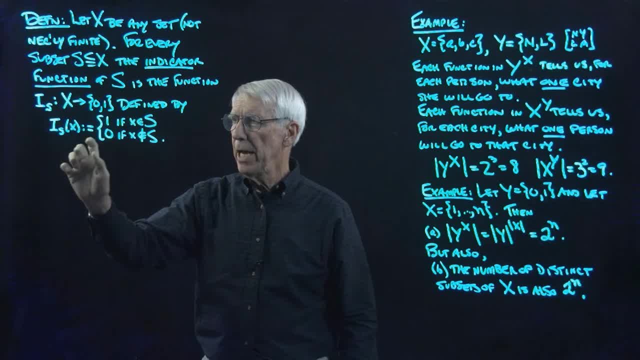 numbers would assign all the rational numbers the number one and would assign all the irrational numbers the number zero. Every single element of x gets assigned a number and the number is one if that element is in subset s and that number is zero if the element is not in s. So let's write down a remark that 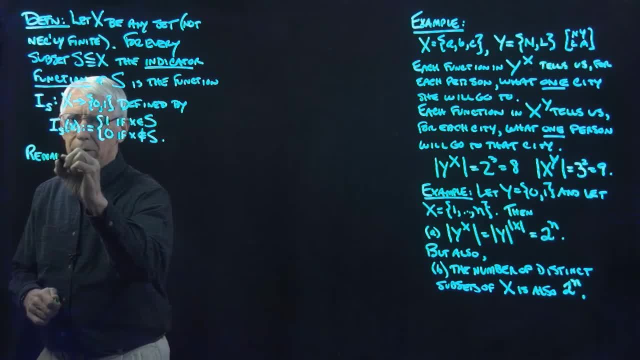 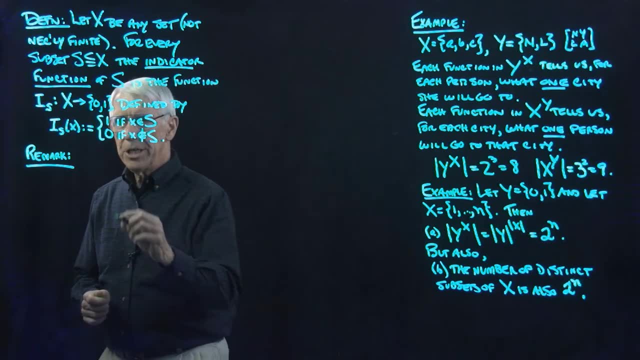 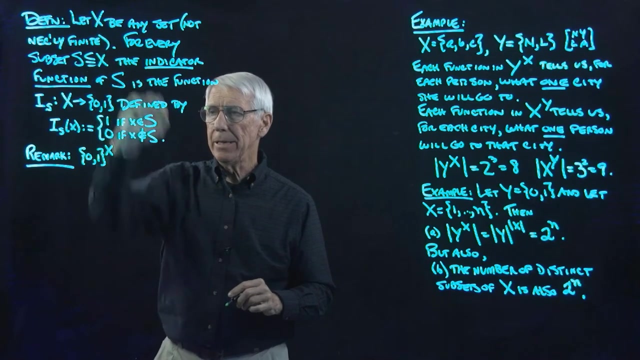 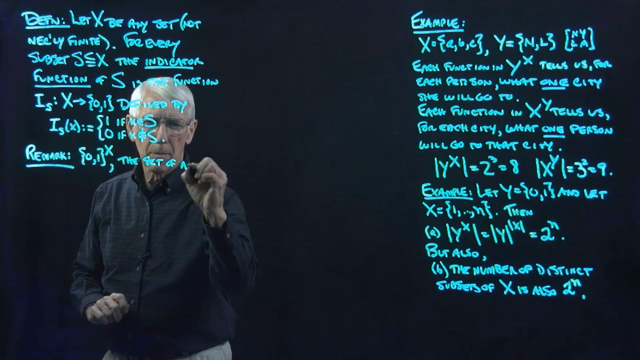 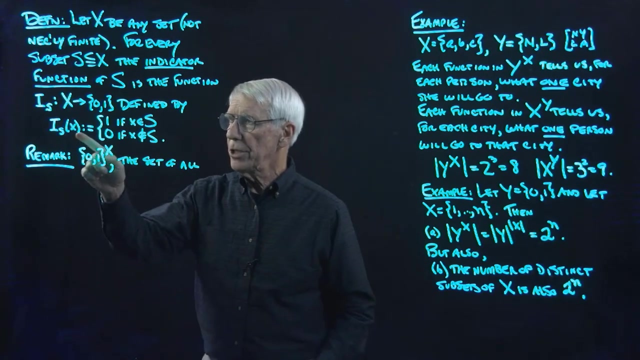 tells us something about this, And that is that zero one, the set, zero one to the x power, where x is a set. So that is the set of all indicator functions, because the indicator functions are functions that go from capital X into zero one. So the functions, the set. 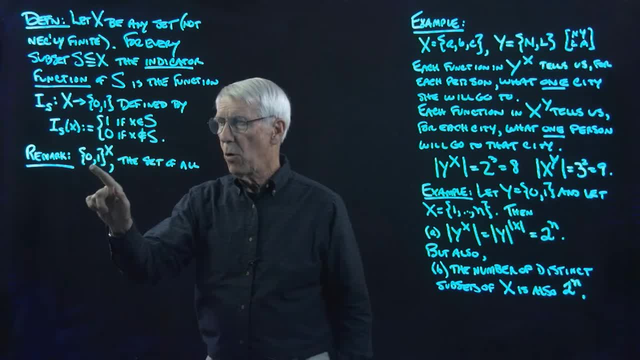 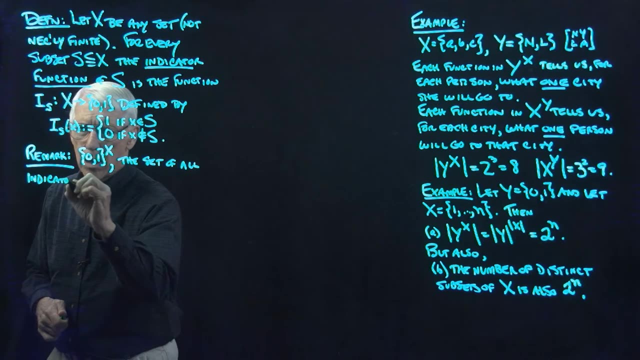 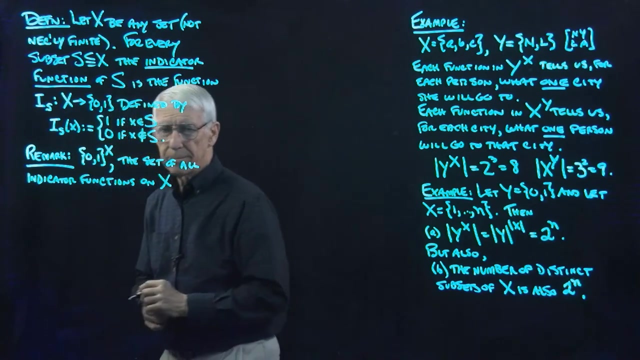 here is all the functions that go from capital X to zero one. So it's all the possible indicator functions, all the functions we can define that assign either zero or one to every element of x. So this is a set of all indicator functions on. x is- and I'm going to put this in quotation marks- is the same as the set. 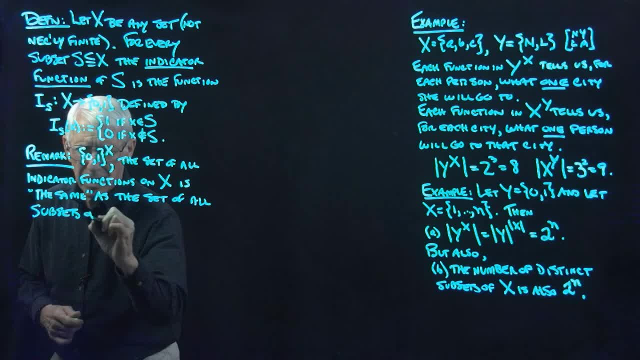 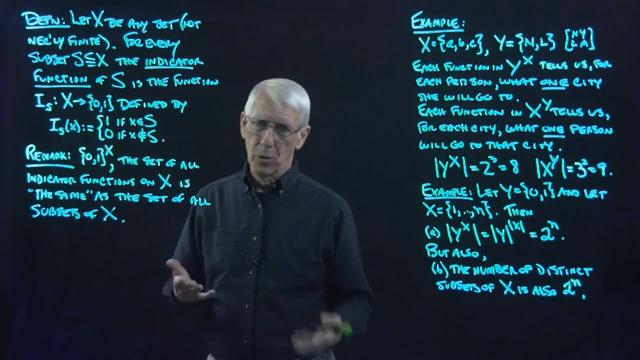 of all subsets of x. Now, what do I mean by the same as Well? what I really mean by the same as is: there's a one to one correspondence between the functions from x into 0, 1.. That is, between the indicator functions and the 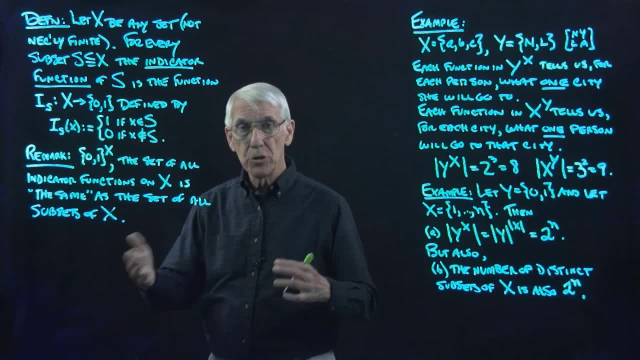 subsets of x, a one-to-one correspondence between those two sets And, in effect, the indicator functions well, in effect. what we're going to do here is we're going to say, in effect, what that one-to-one correspondence is. So let me. 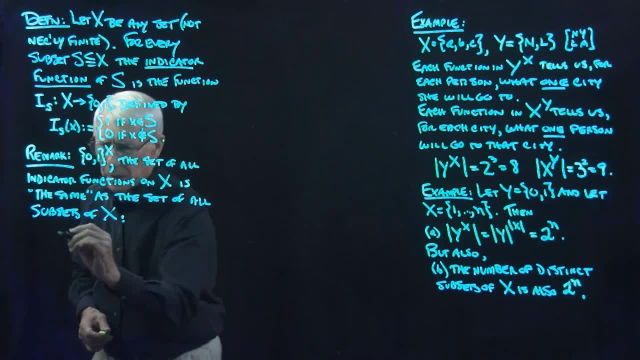 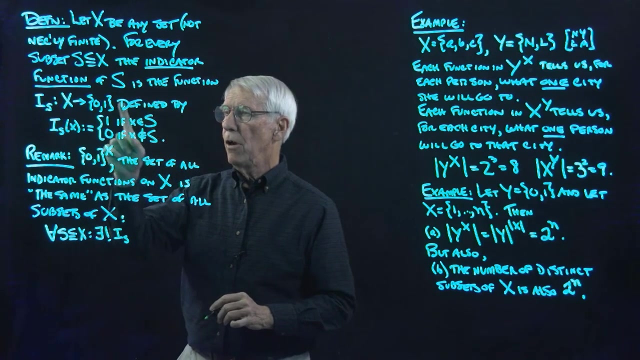 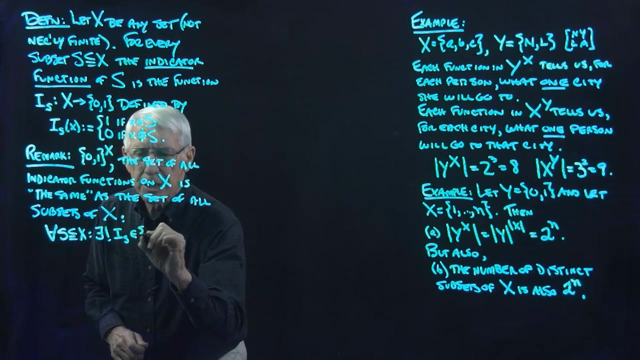 write this with a colon here and say: for every subset of x there exists a unique function. i sub s the indicator function for that set in the subsets set 0,, 1 to the x and for every function, f in the set of functions from x into 0,. 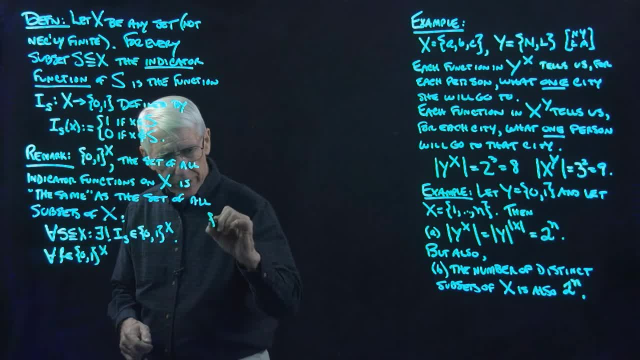 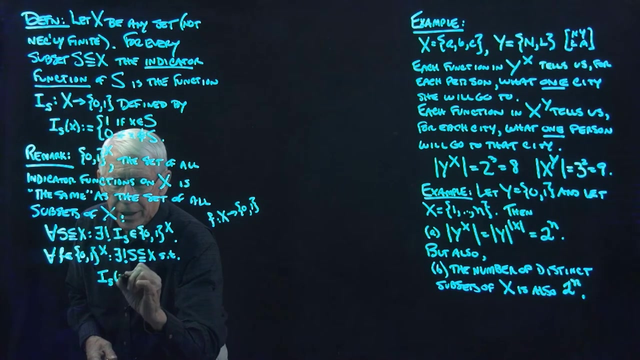 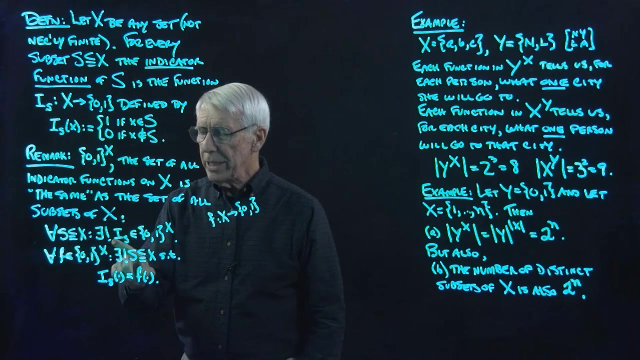 1, that is, every function that goes from x into the set 0, 1,. there exists a unique subset S of x, such that the indicator function for that set is the function f. So let's just kind of review that. It says that given any subset of x, there is a unique. 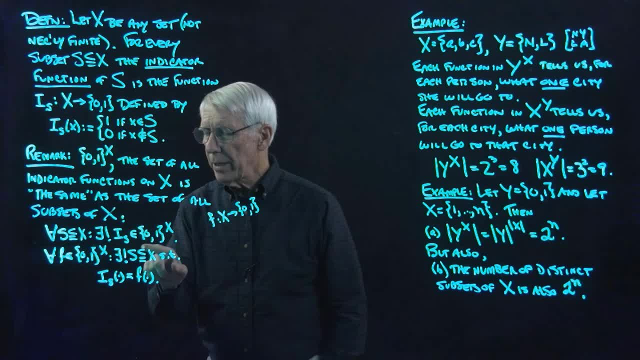 function from x into 0, 1,, which is the indicator function for that subset. Conversely, for any function from x into 0, 1, there is a unique subset for which the elements are exactly the same. So that is, exactly the ones that get assigned 1 in this function and the elements in the 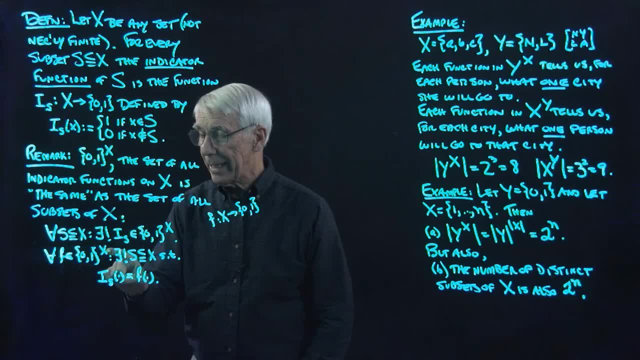 complement of x are exactly the elements of capital X that get assigned the number 0 by this function. In other words, for any function from x into 0, 1,, there is a unique subset of x whose indicator function is that function. So that is so we actually have established. 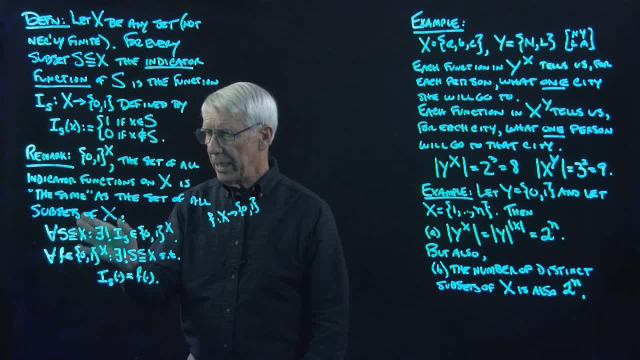 here a 1 to 1 correspondence. So we have a set of x and a subset of x between the indicator functions on x, the functions from x into 0,, 1, and on the other hand, the subsets of x. And so, because of this, 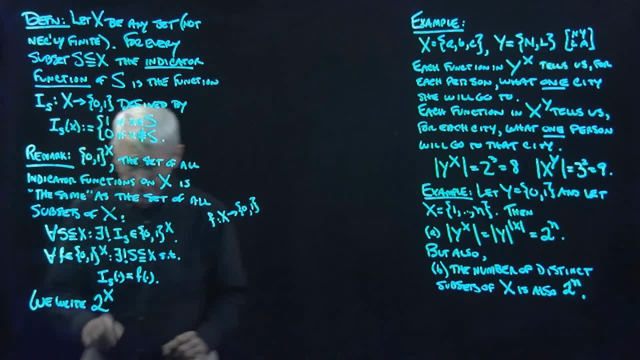 we write 2 to the capital X. well, that's a set, that's a number, that's a set, but this is really just a notation. We write 2 to the x and we write 2 to the x, and we write 2. 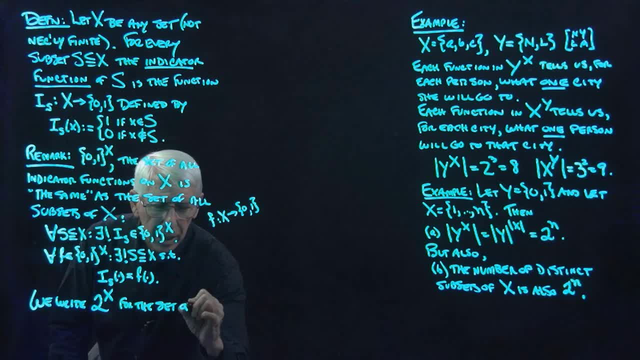 to the set of all subsets of the set x, And we call that the power set of capital X, to give it a name. And I should add that the set of x is the set of x. So the set of x is the power set. 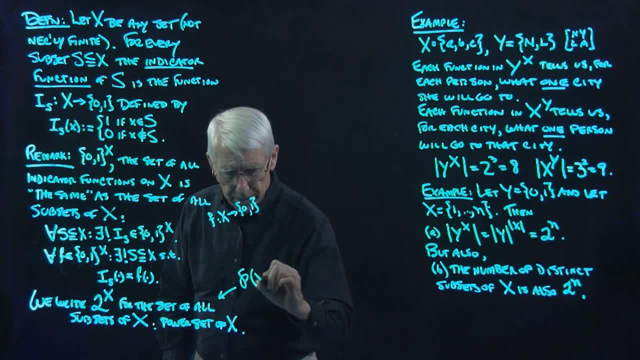 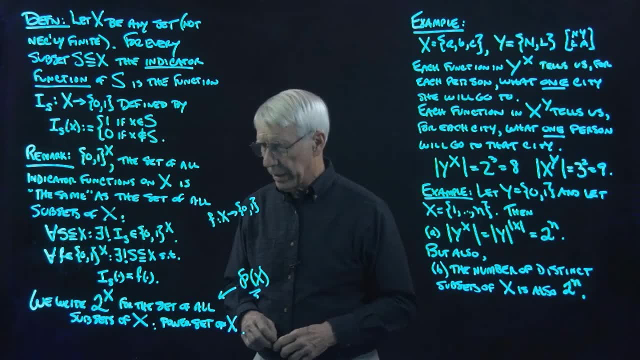 of x And we like to find that here. so we make this set of x and we make that set is sometimes by some people written as the power set of x And I have suggested that. one of the things that you read is parts of the book by Hammock called Book of Proof. 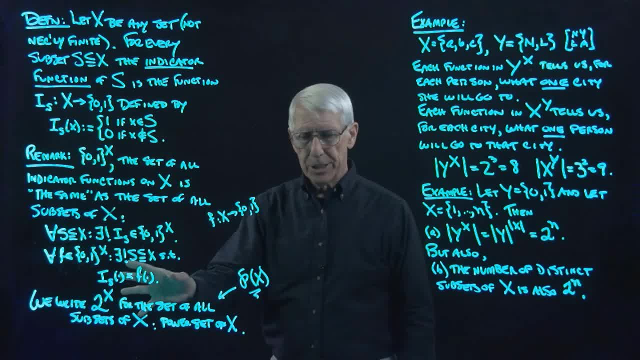 And in that Book of Proof he has all these ideas. He uses this notation. He does not. well, I shouldn't say he has all these. I'm not sure. I don't recall for sure that he has the notion of indicator function. I'm not positive about that. He uses this notation. 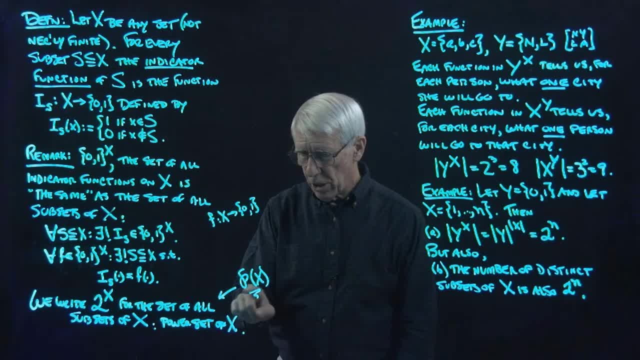 this terminology the power set of x is the set of all subsets of x. He uses this notation for the power set of x. You can see p for power. But I kind of like this notation better because it kind of brings out this unification between subsets, between functions. 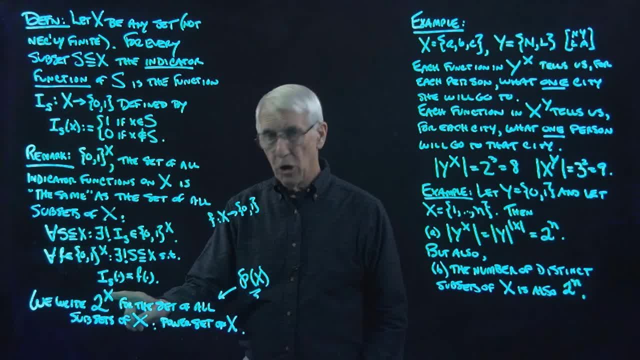 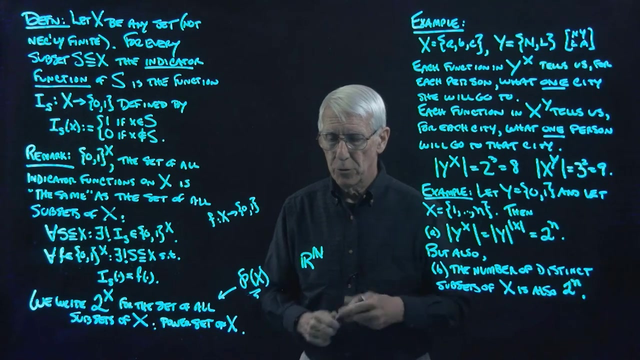 and also between sequences, because of course sequences in x, let's say sequences in r, for example, they're functions from the natural numbers into r. So again like this, And even n-tuples where we could say rn, The set of all functions. 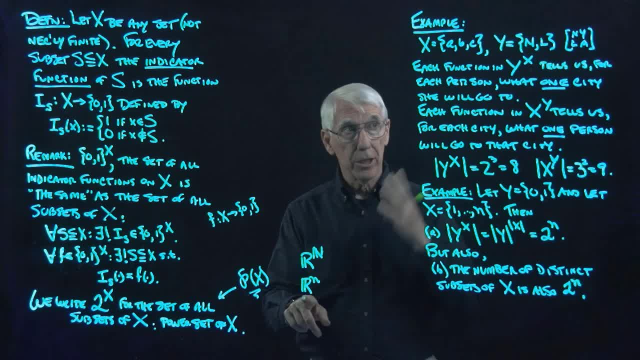 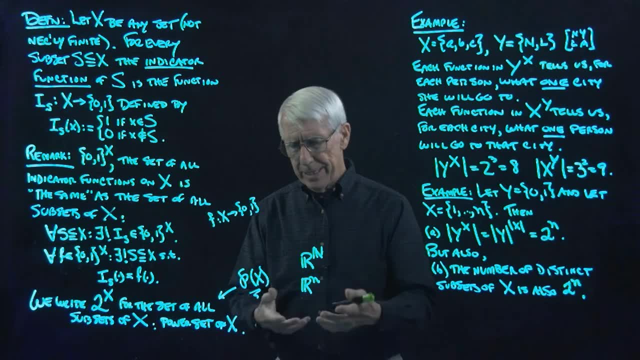 So here we have unifications from an n-element set into r, as we said earlier. So this kind of brings together the ideas of n-tuples, sequences, functions, indicator functions in particular, and subsets of a set and the set of all subsets of x, of any set x. So I think 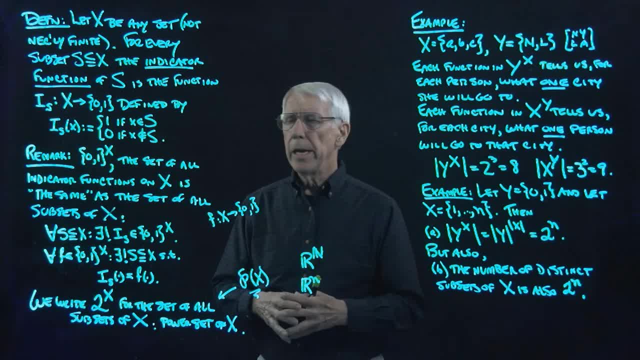 this unification is kind of instructive. Is there another question, though, about this one productive. it's useful. it's a helpful way to kind of get a handle on thinking about these alternative concepts. So that's it for today. See you all next time.